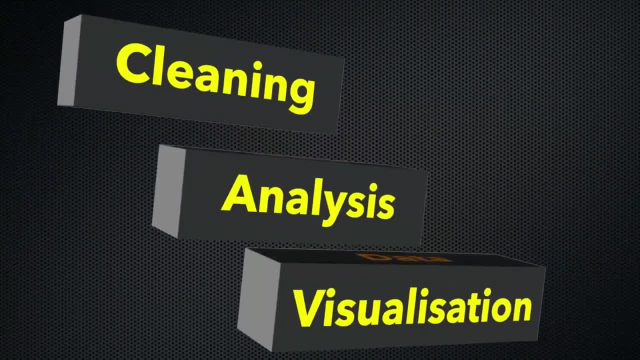 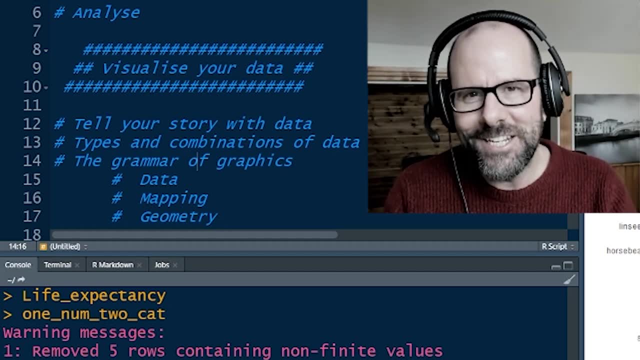 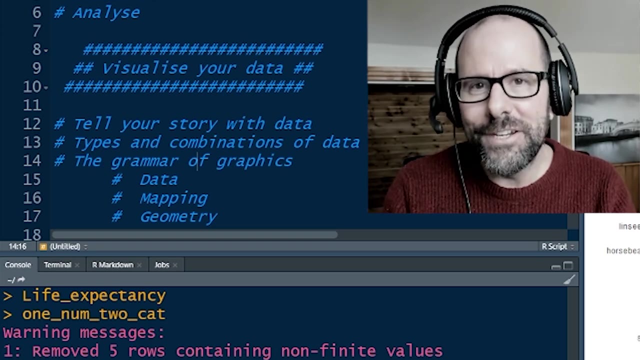 videos on everything. Now, all of the code that I use in this video is available to you right now on a cheat sheet. I'm going to tell you at the end of this video how to download that cheat sheet and you can replicate everything that I'm doing and experiment with it and improve on it. The data that I use in this: 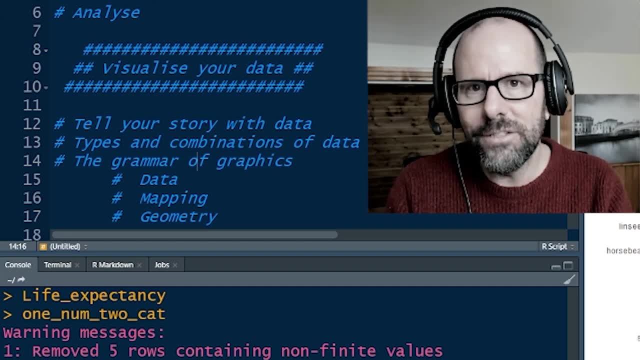 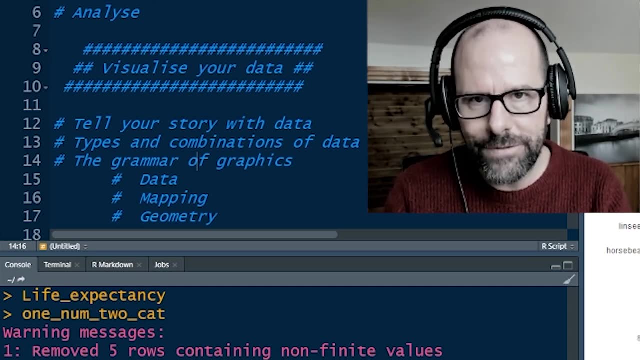 video is also available. It's actually on your computer right now, right? So R has got built-in data sets that you can use to practice, and those are the data sets that I use in order to produce the graphics that I do in this video. So there's no going and fetching data or everything that I'm 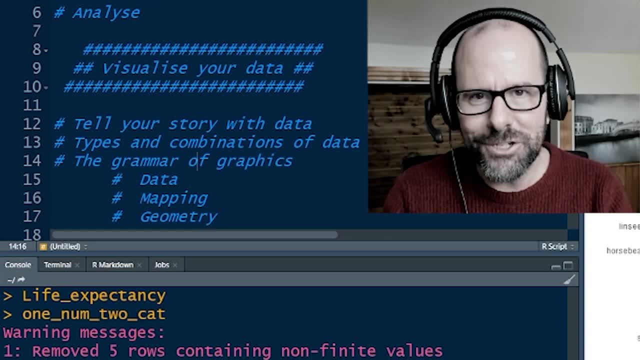 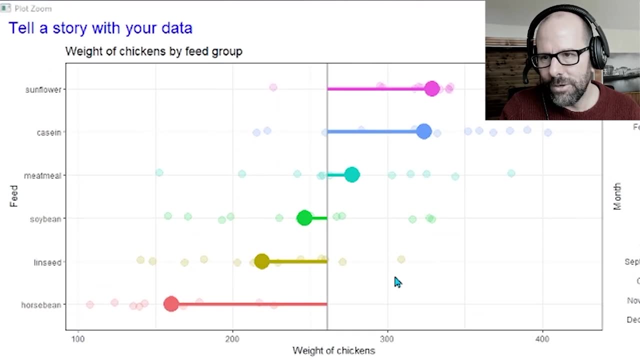 doing You can do at home. replicate it, do it better. Let's keep going. I just want to use these plots to illustrate the fact that you can use data to tell a story. right Top, left-hand plot: this is weight of chickens by feed group. Each of these are feed groups and the big dot is the. 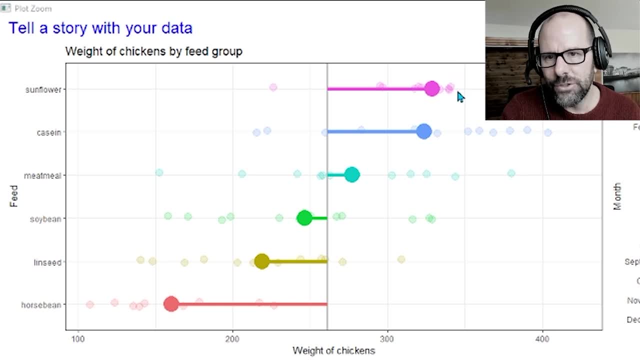 small little light dots are each observation, each individual chicken, their weight. The big dots are the average weight within that group. This line down the middle is the average weight for all of the chickens. You see that these three over here are above average. These three over here are below average. 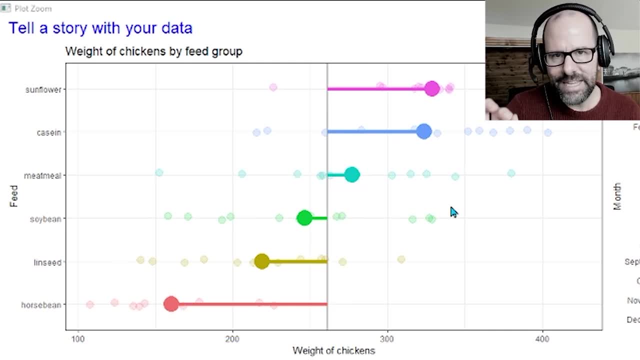 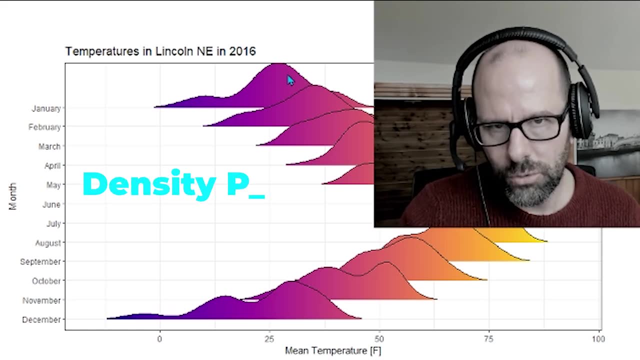 and you can see which are on the extremes- Tells a story. Looking at the graph, you immediately know what's going on. This graph is all about temperature and each of these density plots- and we'll talk more about what a density plot is later on in this video- Each density plot, 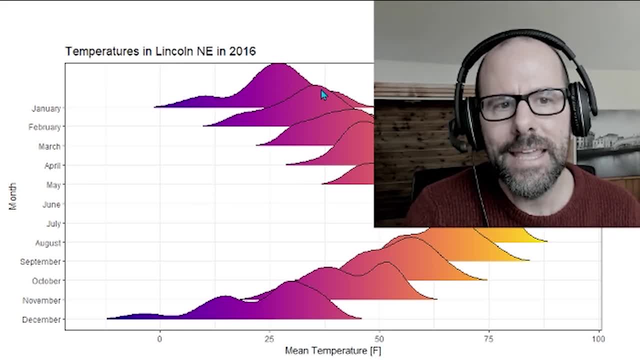 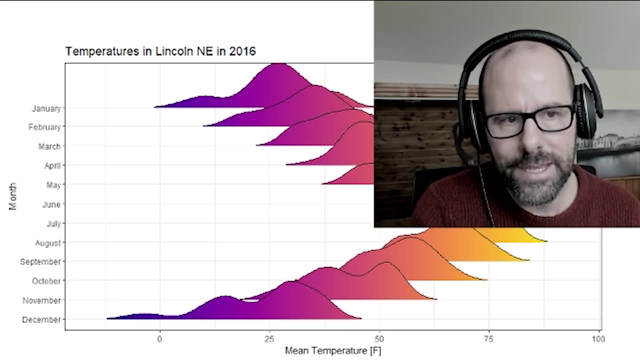 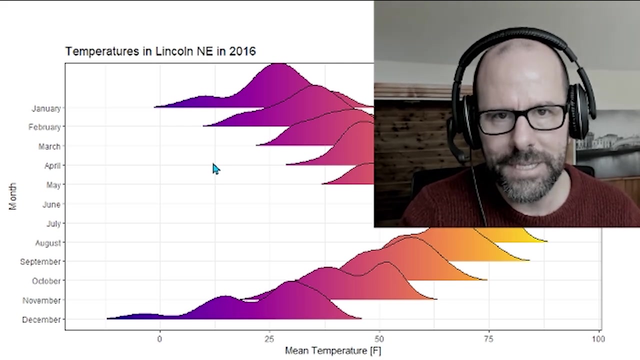 represents the distribution of temperatures in a given month in the year 2016.. Now then we compare month on month and we can see that the density plots themselves. So the more you have long and everything gets warmer. we also use in color here to represent temperature. So the more to the right you are, the higher the temperature, the more the color turns kind of yellowy, orange, right, And you can immediately see as the year unfolds. we go into the summer, everything gets warmer, And then obviously things get colder during the winter. And during a month you can also see the same thing applies. There's this distribution of temperatures. Easy to see what's going on. It tells a story, It jumps off the page. You know exactly what is going on. right, You got it. Yippee-ki-yay, Let's keep going. 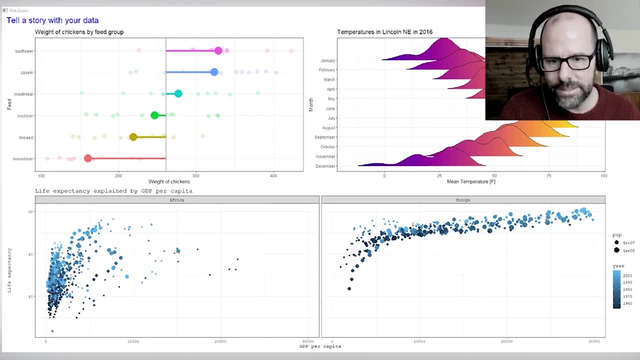 So the density plot down here uses five variables. right, We've got a lot going on here. These two things here are two facets of one plot, So everything at the bottom is really one big plot. Okay, what have we got going here? We've got: life expectancy is the dependent variable. That's a function of something, Something's affecting life expectancy here. We've divided it into Africa and Europe. And the independent variable, the thing that we think may have an effect on life expectancy, is GDP per capita. In other words, how? 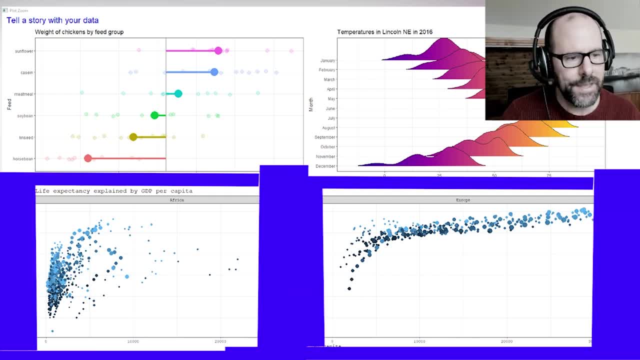 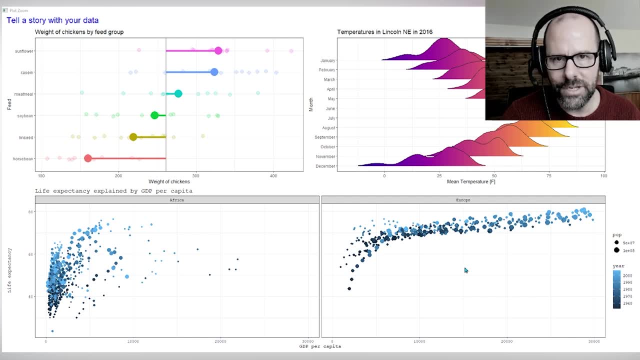 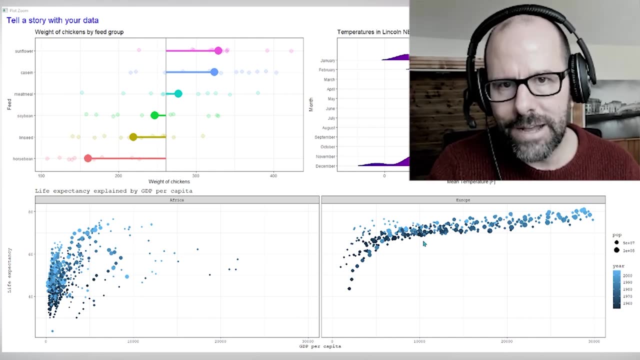 each of the dots is a country, The color of the dot tells us what year that we're talking about that dot is from, And the size of the dot tells us the size of the population in the country at that point in time. And, of course, we divide it into Africa and Europe. So think about what we've got here. We've actually got five variables. We've got one categorical right, And it's выход table. 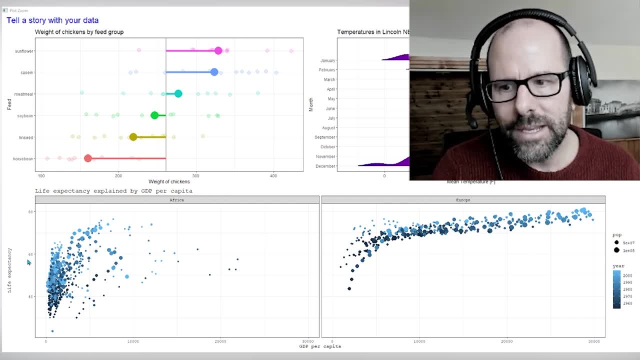 right, And it's not a continent. So Africa and Europe, And then we've got four numeric: life expectancy, GDP per capita, year and population size, And we've got a function of something called this as well. So, if asked, the given count tells us what year that we are talking about. It says: 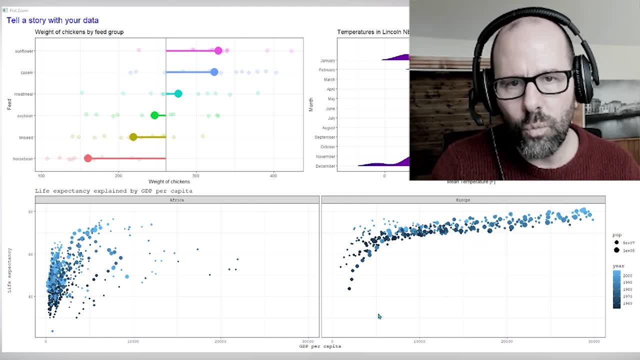 Greg tailed it. Yeah, so we're representing five different variables on one plot and it's very easy to see what's happening here. we can see that as gdp per capita goes up in africa, there's a dramatic increase in life expectancy. you see the same thing happening in europe, but it's a much shallower curve all. 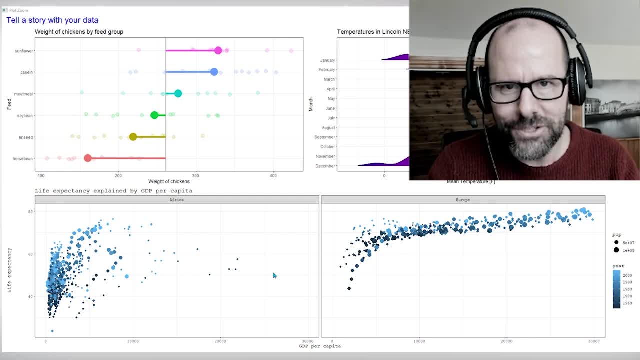 right. so the underlying message, the underlying story that you're telling jumps off the page, easy to see and it's absolutely beautiful. right, you got it hot diggity. let's keep going. okay, stop watching the video. stop watching the video. i want to give a quick, big thank you to 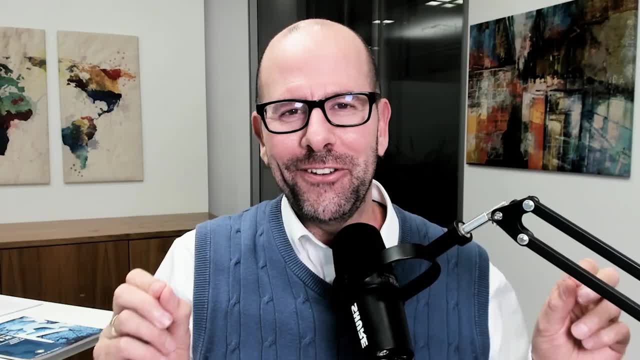 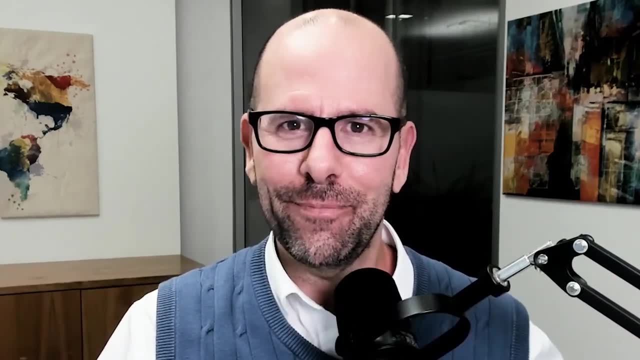 nested knowledge for supporting the creation of this video. if you've ever gone through the struggle of doing a literature review or a systematic literature review, believe me i know your pain. i've been there and what i'm about to tell you is going to absolutely blow your mind. 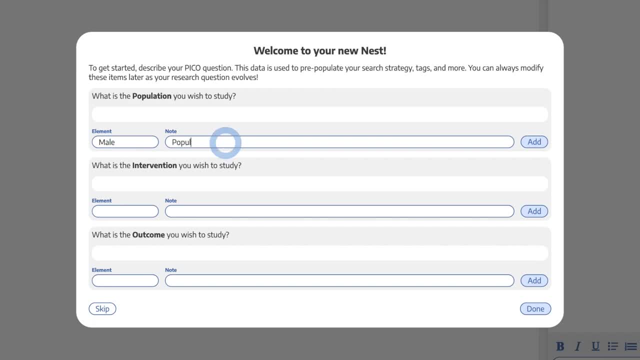 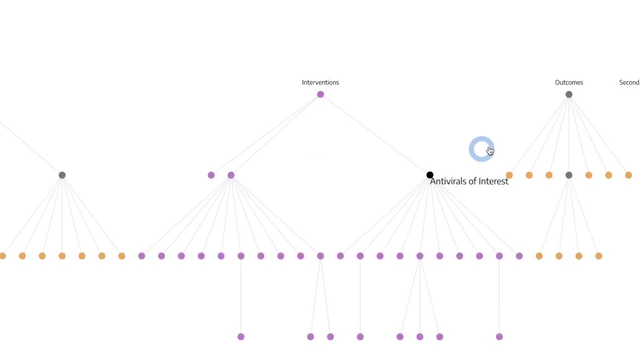 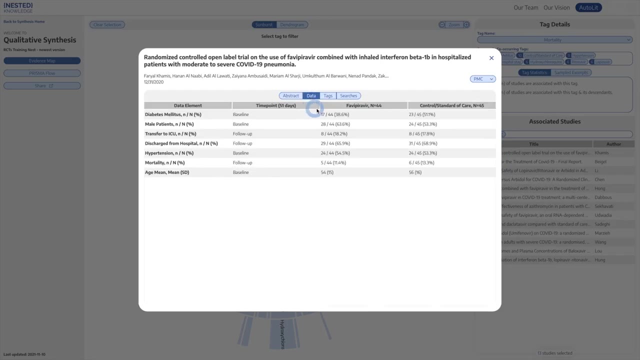 nested knowledge have a platform that supports the entire process, from designing your research question and search parameters to screening, tagging and extracting the appropriate parameters. the platform automatically generates visuals that you can use for qualitative analysis, so check out these interactive sunburst diagrams used to get an overview of trial endpoints or 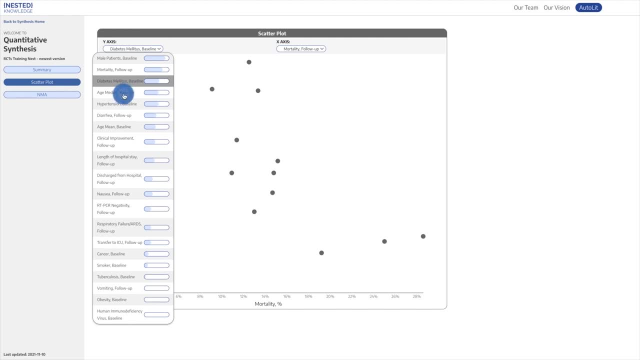 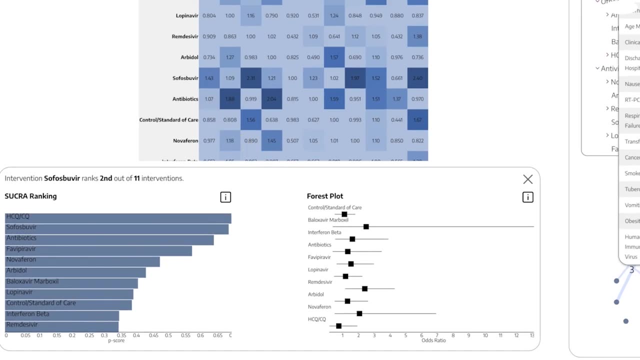 and this is going to blow your mind. it can extract study results to do meta analysis. so check out these ready for publication forest plots. and this next amazing feature is going to become, i believe, the new standard for systematic review. it's being able to publish a living document that auto. 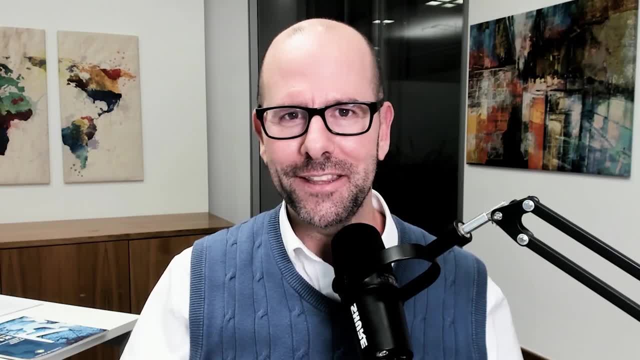 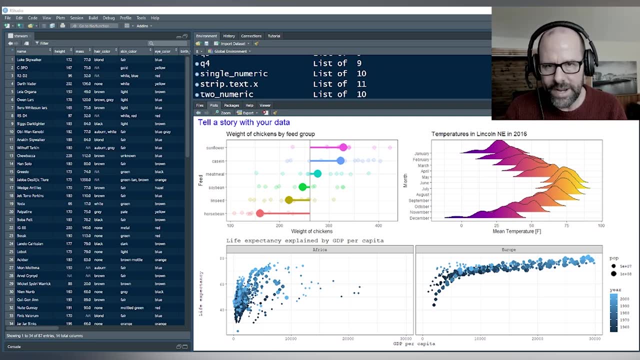 updates as more data becomes available, so check them out by clicking on the link in the description below. okay, let's get on with the video now to understand what graphic to use with what plots to use, when we're just going to have a look at different variables and different combinations of. 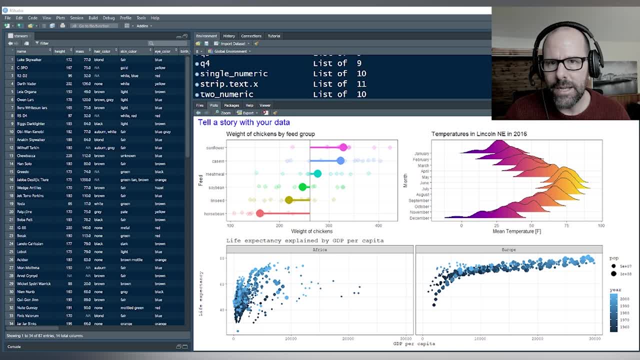 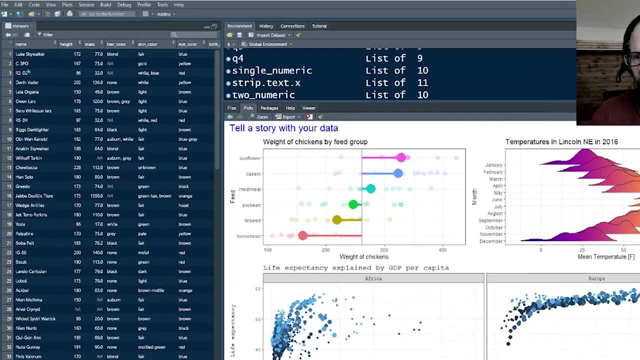 variables. and to do that we're going to take a look at the star wars data set now. this data set is on your computer right now, so you can. you can view it and i've put it up on the screen over here and we see, we've got all the star wars characters and then we've got a number of variables. we've got 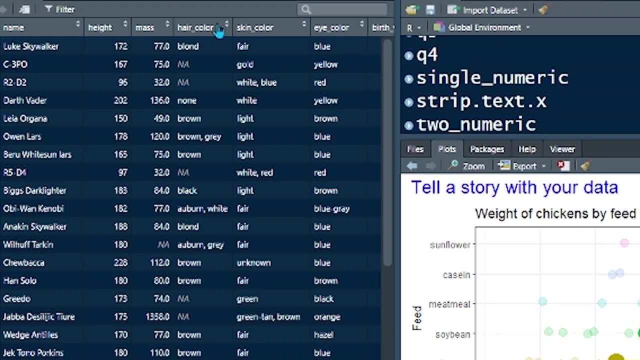 some numeric. we've got some categorical variables right: height, mass, hair color, skin color, eye color, etc. etc. we're going to mostly use a height mass. i think. we're going to use hair color and we're going to use gender as well, okay, and we're going to look at combinations of categorical and numeric. 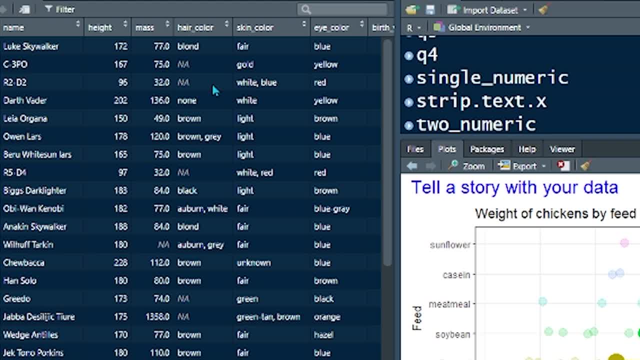 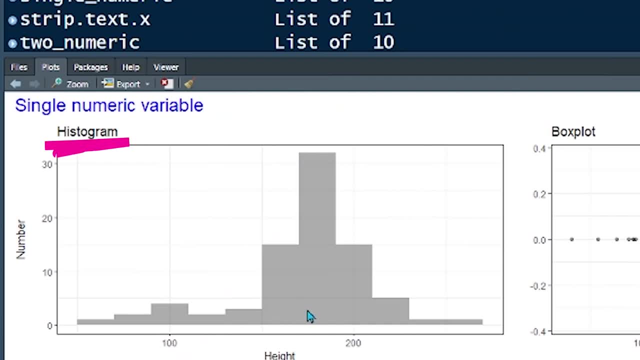 variables and decide what kind of graphics we can use to represent those. we'll start off by looking at a single numeric variable, in this case height. typically we might use a histogram. the data is put into buckets or bins and for each bin we count up the number of observations and that is represented. 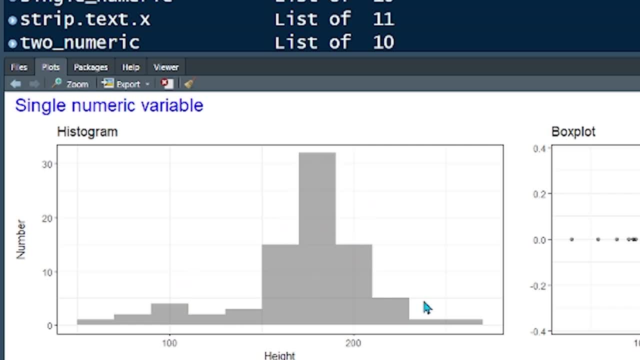 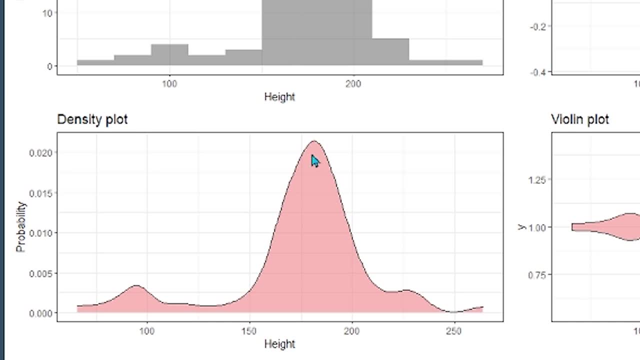 by the height of the column right, so we get a sense of the shape of the data. similarly, a density plot right is basically the same idea, except it's not a count of the number of observations, but it's really the probability of an observation at a given height. in this case, 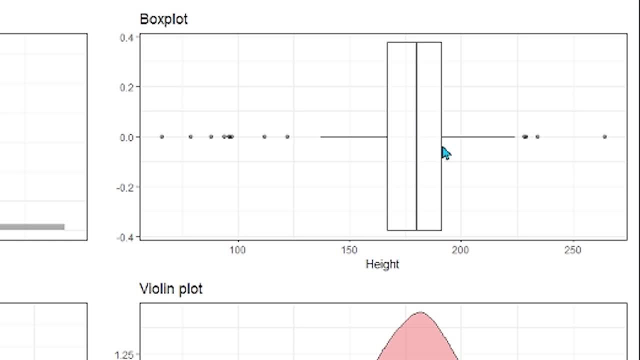 box plot tells you about the distribution of the data. so the box itself represents 50 of the data. the line in the middle is the median. these little whiskers are 1.5, the interquartile range, and then everything else is an outlier. and a violin plot is very much like a box plot, but 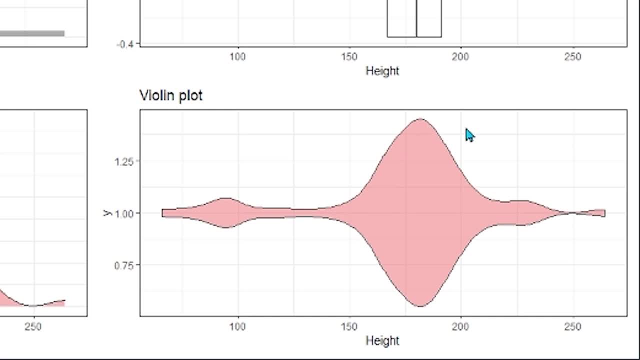 it's more of it's. it's similar to a density plot as well, in the sense that it's just a bunch of data, but that's the distribution and you can see the shape of the data. these. these are often more useful when we're looking at data that's been then disaggregated by. 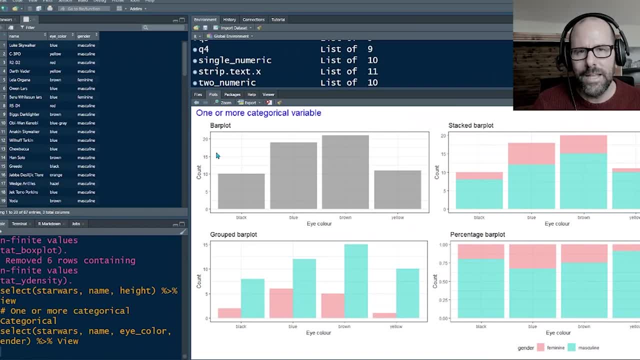 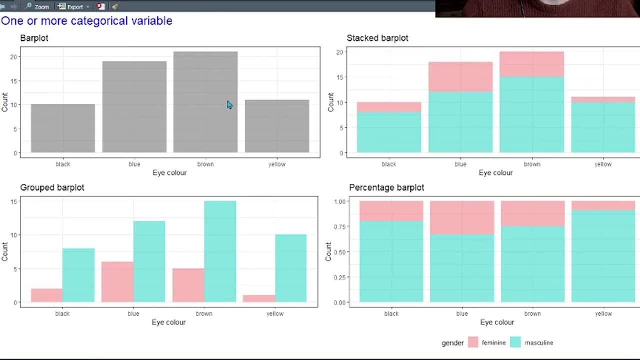 a categorical variable and we're going to look at that later on in this video. now let's look at one or more categorical variable. very straightforward: here we've got eye color and gender. if you're just looking at one categorical variable, a bar plot is perfectly, perfectly fine. 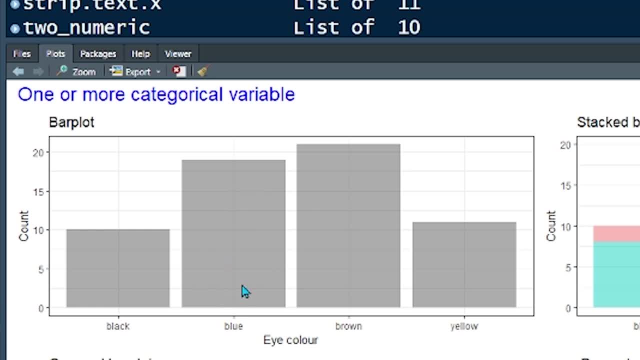 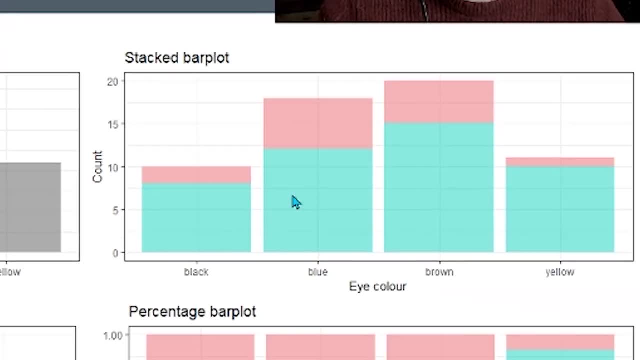 and each bar is just the height. it's a count of the number of observations in each category. once you add in another category, you can disaggregate these bars by the new category, in this case gender- masculine and feminine- and we've used color to just just to divide up what. 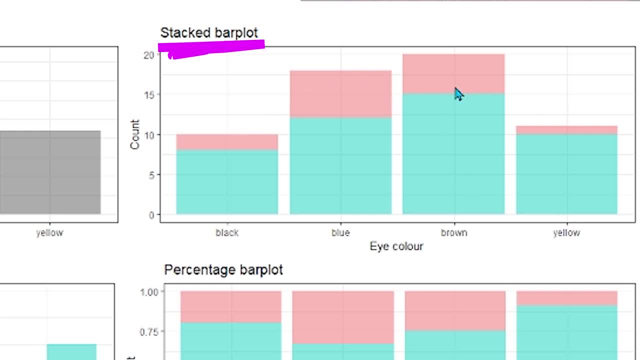 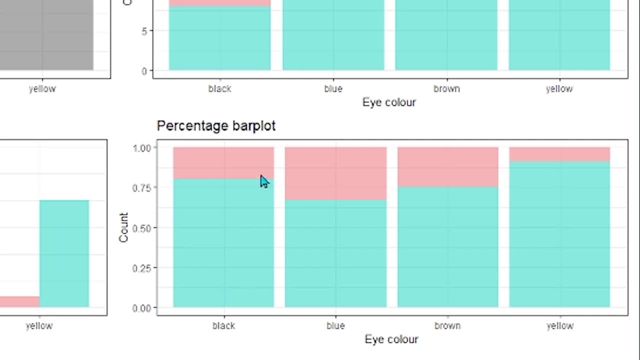 the bars are made up of. so this is a stacked bar plot. you can have a grouped bar plot where you've disaggregated and you've put them next to each other, and a percentage or proportion where they all add up to one or add up to 100 and you can see the relative contribution. 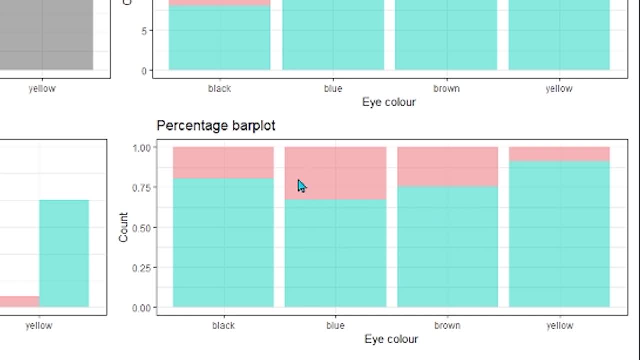 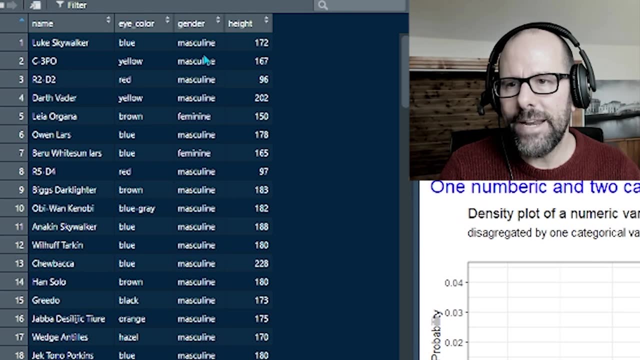 of each of those categories. okay, super duper easy, let's keep going. okay, in the last example we had eye color and gender, but now we're adding in height. so we've got two categorical and one numeric. okay, let's talk about how we'd represent that. very often, once you introduce a numeric, 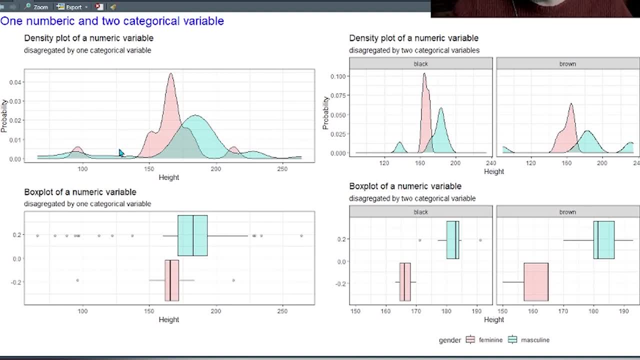 variable into into play. the numeric variable really drives what the geometry is. in other words, in this case we're looking at density plots- you could use histograms. we're looking at at box plots, but you could use violin plots. but the actual geometry here has been driven by the numeric variable and we're using the 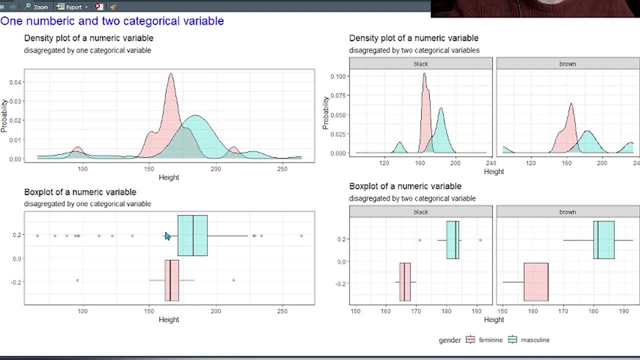 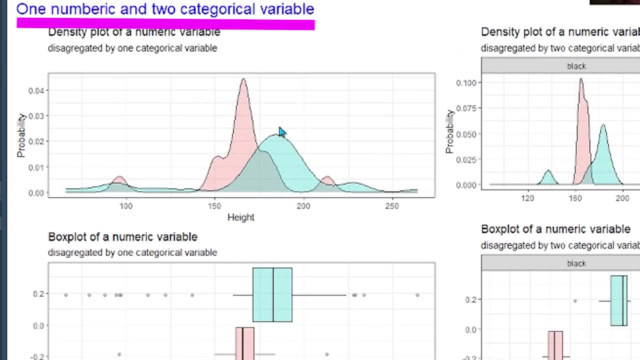 categorical variable to disaggregate that data, to disaggregate those graphics. okay, and let's look at what we've done. here we've got a density plot of one numeric and two categorics. here we've just got one numeric and one categorical right. so we've got height and we've disaggregated it. 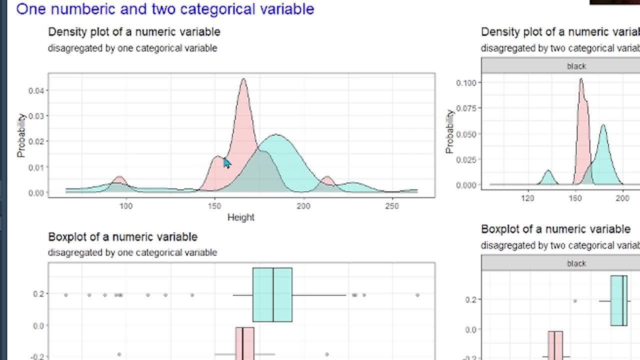 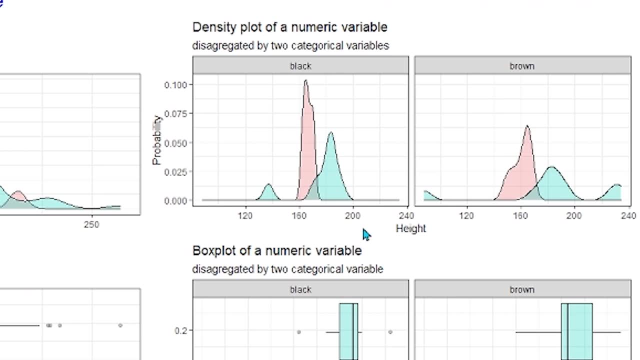 in this case by by gender right. so we've got pink and blue right. same with the box plots: same idea, but we can disaggregate it further and in this case i've we've got eye color built into it, so we've got colors. are being used to represent the different density plots and then facets are used. 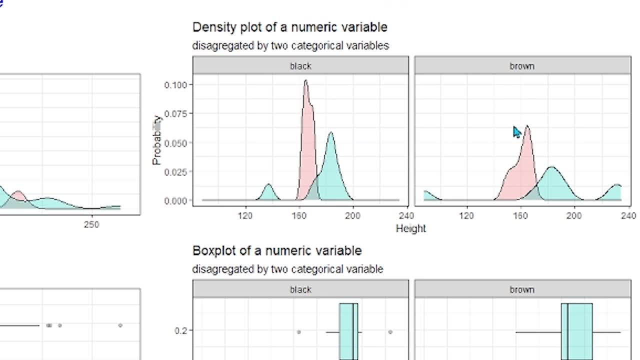 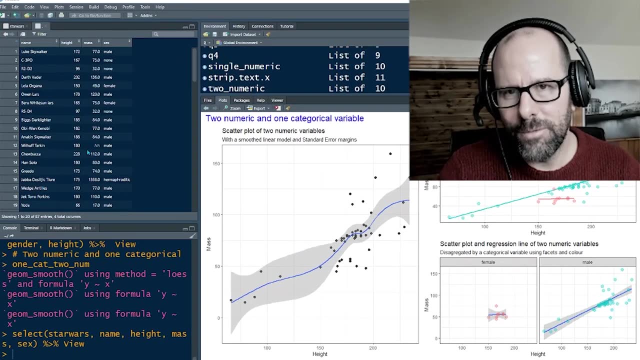 to to divide it out even further in terms of eye color, right, and we've done that with density plots and with box plots over here. okay, super duper easy, let's keep going. in the last example, we looked at two categoricals and one numeric. what about if we had two numerics and one categorical? 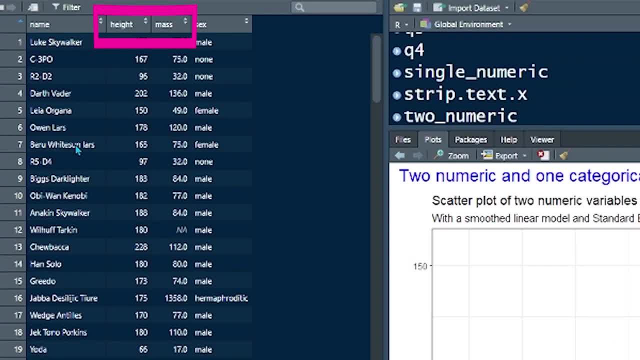 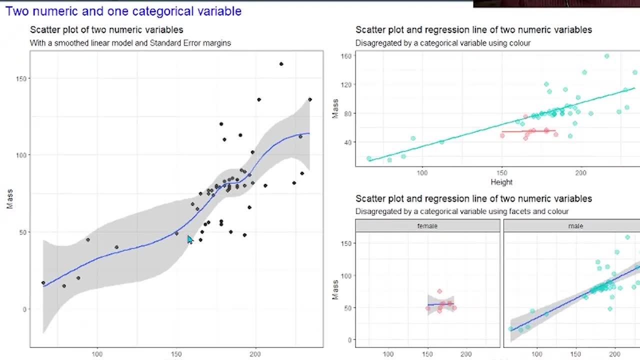 so we've got height, we've got mass, right, two numerics and then one. i've used sex instead of gender, it doesn't really matter. okay, let's look at the graphs. in the first graph, basically, i've just shown you two numerics, right? so before, before, before we, before we build into what to do with the 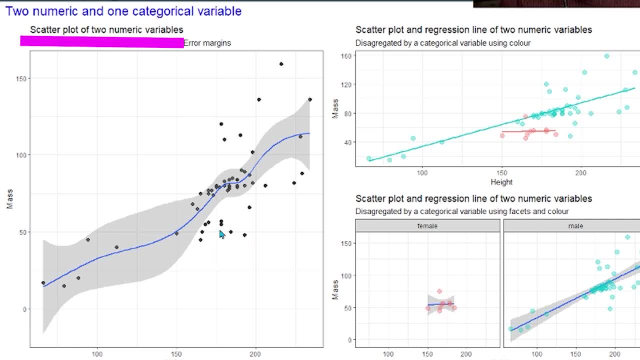 categorical. okay, two numeric variables, scatter plot. we just basically each observation represents for that observation what the mass and height were. we can see there's a nice relationship here. just for the sake of showing you, i've put in what's called a smooth interval into that with with standard errors around that. it's a nice way of seeing what's. 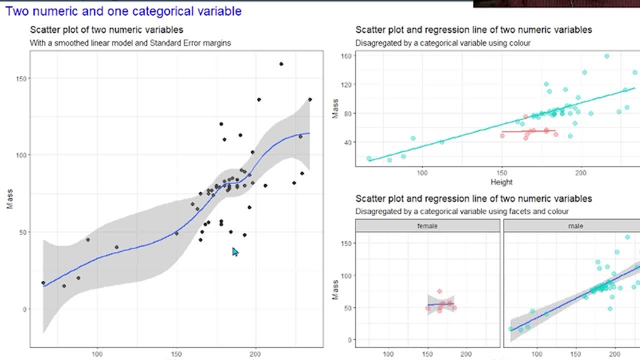 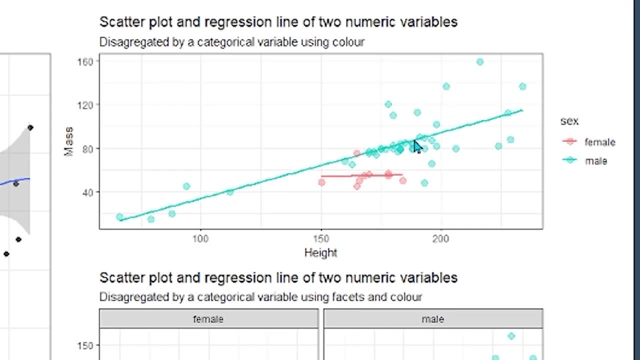 going on in with the data. right now, when we add in sex, in this case male and female, we can disaggregate all of those data points by giving them their respective colors, based on mapping the color out against that particular variable- sex, male and female- right, and we can see that. 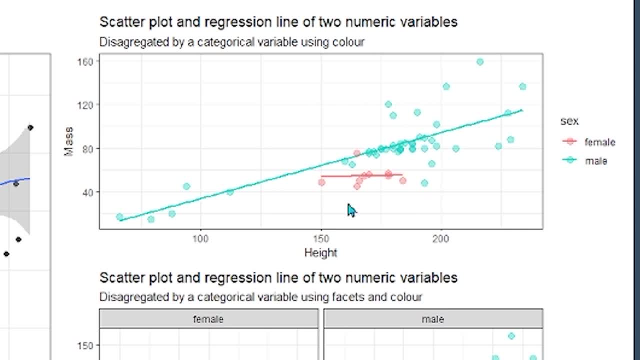 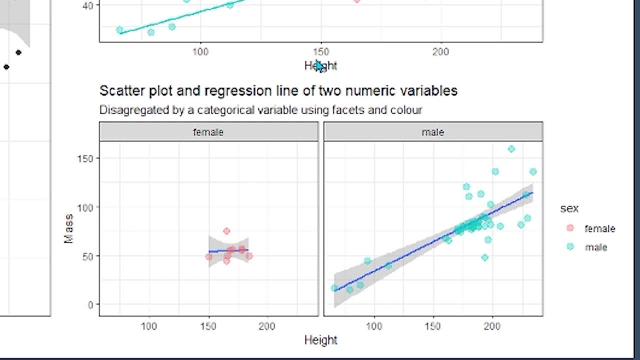 we've divided it up on one, on one canvas, or you can divide the canvas up into facets and look at females and males separately. okay, super, duper, easy, okay. so we've got a nice enough number of things there and we've got a nice enough number of things to do. let's keep going. 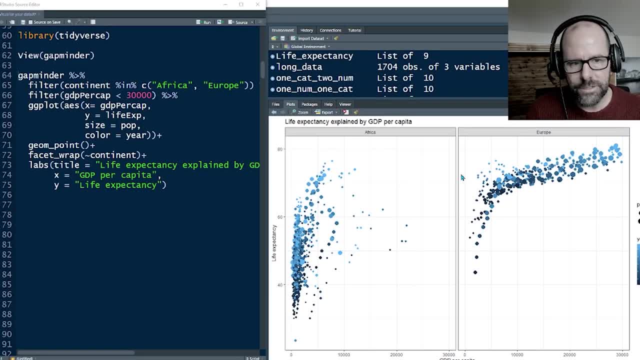 okay, i'm going to talk you through the code that i've used, and it's not much. it's very easy to produce this graphic that's on the screen at the moment. it nicely illustrates how ggplot works and how the grammar of graphics works right. so if you understand this, you'll be able to understand. 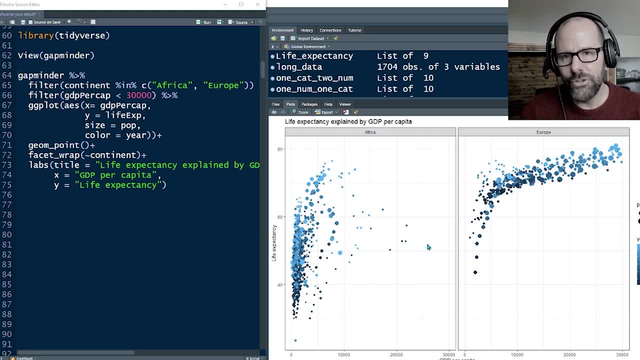 the code that you can download in the cheat sheet that i'm going to tell you about in a minute. you'll understand all of that code because it all follows the exact same principles right now. we said earlier on that basically, the grammar of graphics is: firstly, you define the data. 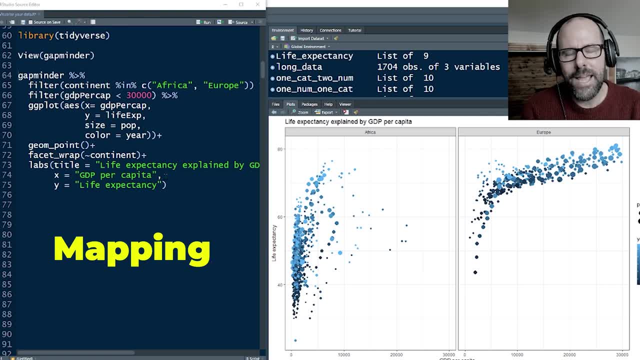 secondly, you define the aesthetics or the mapping, and then finally, you just define the geometry, right. these, those are the three components, and then you can add stuff to it afterwards, the theme, and you can do a few things after that. you know there's, you don't stop there, but that those are. 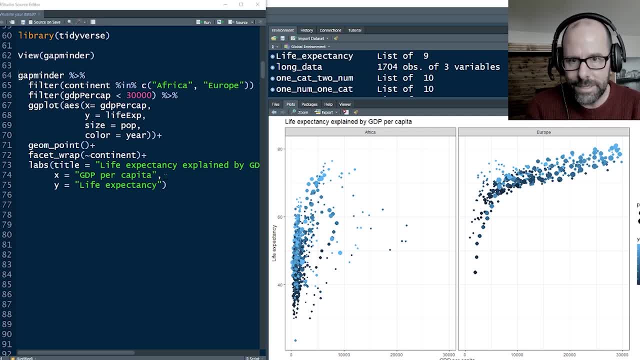 the three principal components right: the data, the mapping, and then the geometry right. and if you've got that, you're good to go. let's- let's look at how i use those three ideas in producing this graphic. first of all, i wanted to get the right data fed into ggplot right, and to do that now you're going. 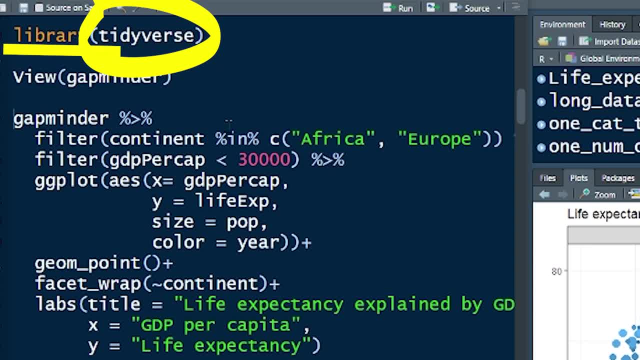 to need to know that you've got all the data up there. so you've got the data. now you've got all the data you want to use. it's not going to be just a simple user guide, but it's going to be a little bit more complicated than you might think. you might be. just first of all, tidyverse, okay. 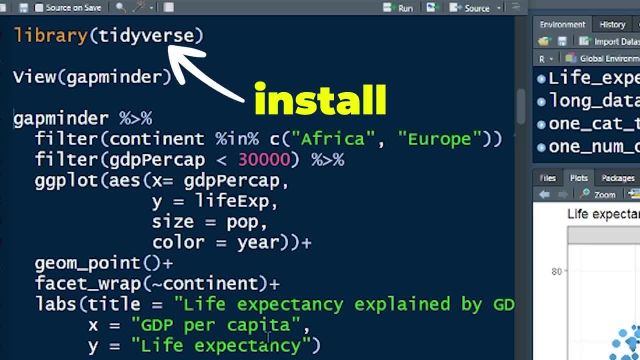 library. tidyverse gets you ggplot and other packages. it brings all of them into play at the same time, so i always use the tidyverse. ggplot comes along with that. uh, you might, and obviously you have to install it first if you've never installed it. install packages tidyverse also. 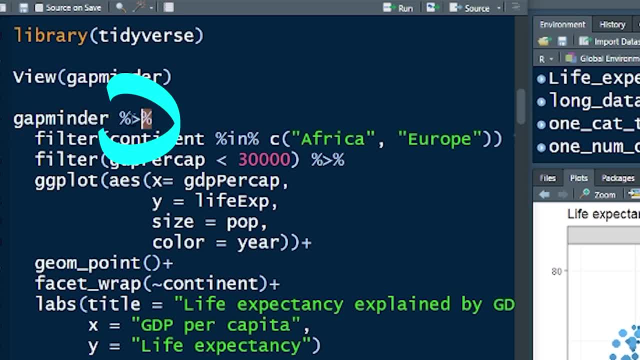 install packages- gapminder, right. and then you want to say library cap- gapminder as well. then the data is available to you to use right now, right. so we start off by saying gapminder. that's the first step, telling us we're using the start. this little pipe operator simply means: and then right, we pipe what? 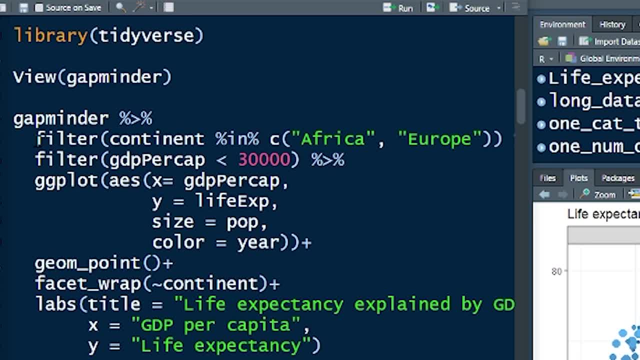 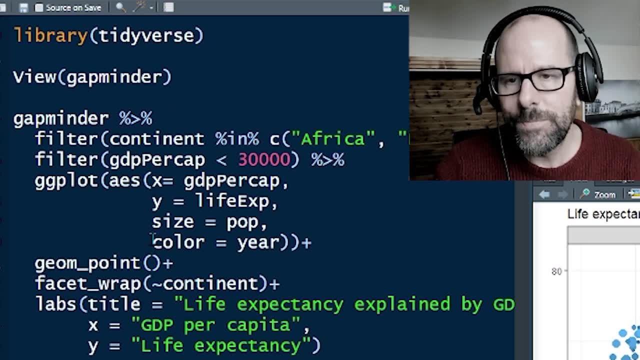 is ever on the left of the pipe into the next line of code, right? i'm not going to try and teach you how to use dplyr and tidyverse in this video. i'm assuming you're familiar with that. i'm teaching you how to use ggplot- right, but what's nice about ggplot is that we're going to use these pipe. 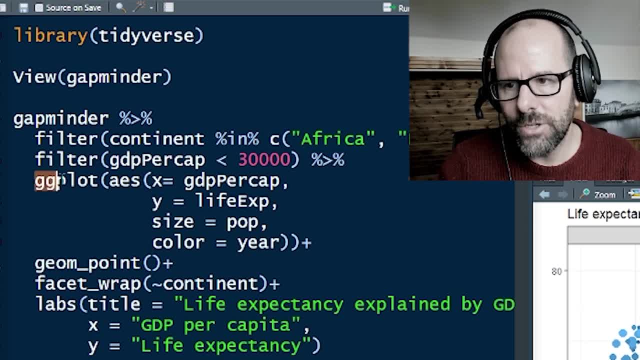 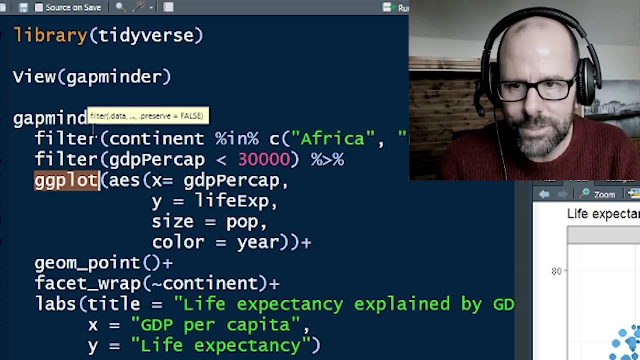 operators to feed into ggplot. here we start with ggplot here to feed into ggplot the exact kind filtered out data set that we want, right, and then? so we can actually manipulate the data. as it's getting fed into ggplot, we can do things to it, which is lovely. that's. that's why this is so. 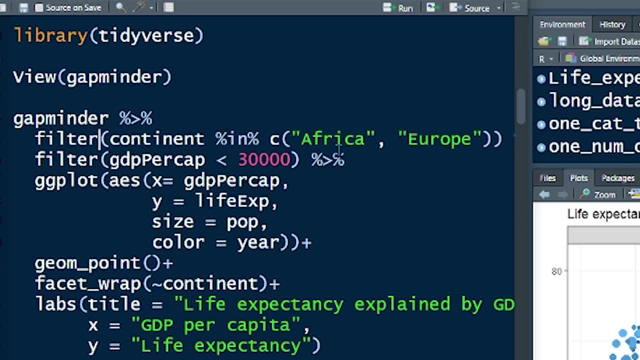 beautiful right. so, first of all, we don't want all of the continents in our data set, so we filter, we say continents in, and this is a concatenation and this isn't a video about how to do filters. watch another video for that if you're confused. but we basically said we're filtering it and we 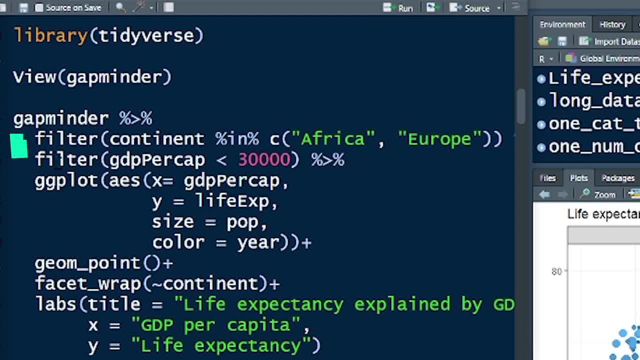 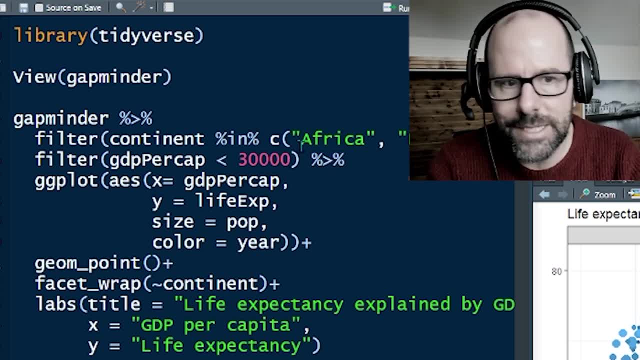 just want, uh, we just want africa and europe. right, then we're doing another filter and we're saying we just want gdp, uh, per capita of less than 30 000. right, that's just to keep. that was just to keep the graphic nice and manageable, and so it's visually easy. 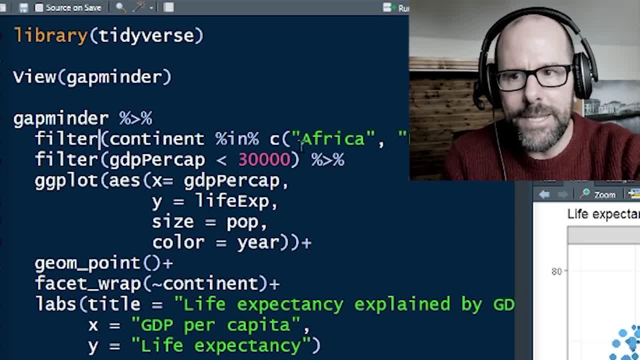 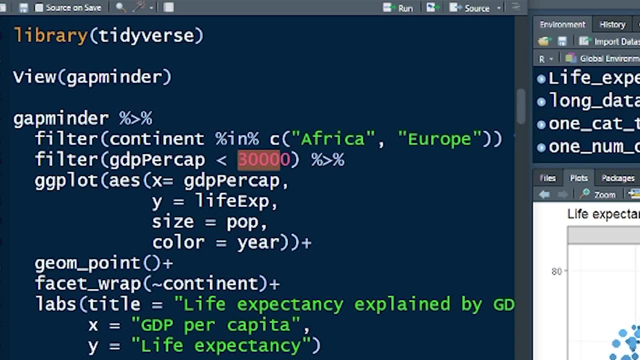 to see what's going on and to show you that you can be manipulating your data as it gets fed into ggplot and and we can make changes. i mean we could. just if we changed this number here, the graphic would immediately change. if we changed the number of continents there, that would change in the 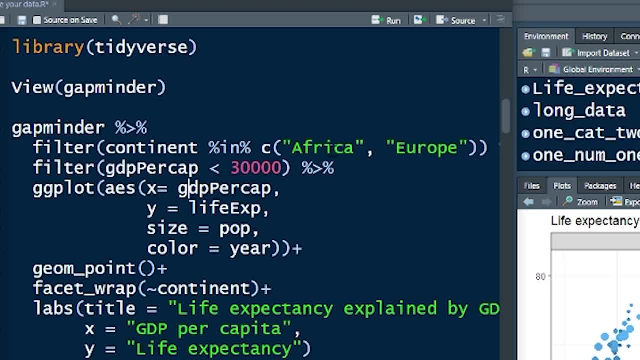 graphics straight away. okay, so that's quite nice. then we're feeding in this new data frame that we've now just defined into ggplot. the first argument in ggplot is usually data right. so if if we hadn't done all of that, i would have been saying data is equal to uh and uh gap minder. 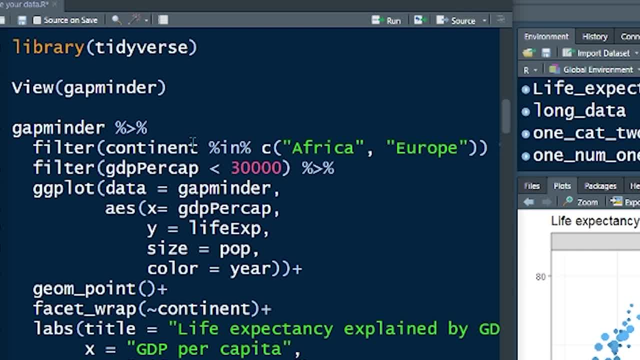 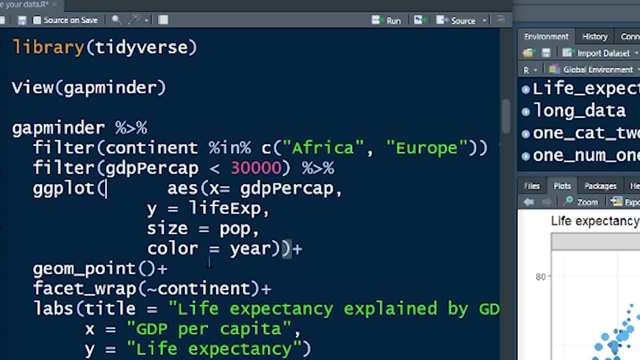 comma, and then i'd carry on. but because we're working in the tidyverse, we don't have to say data is equal to that, because we're feeding the data in with the pipe operator okay, so that doesn't apply. um, similarly, here's a little bit of a different way of doing this. we're going to say: 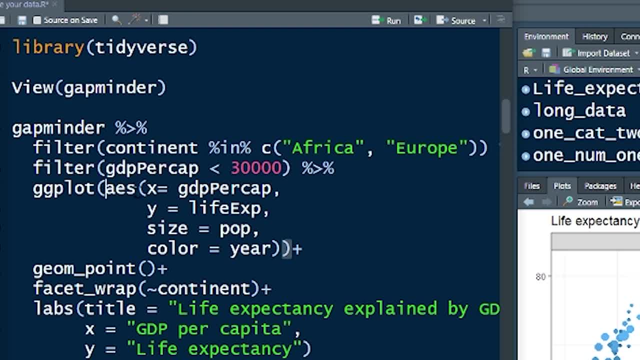 similarly here we're just starting with with the word, with aesthetics. but really what? what you don't need to type, but what's happening in the background is this is mapping is equal to aesthetics. but you don't have to say that right, that's just, it's assumed right. so we just say: 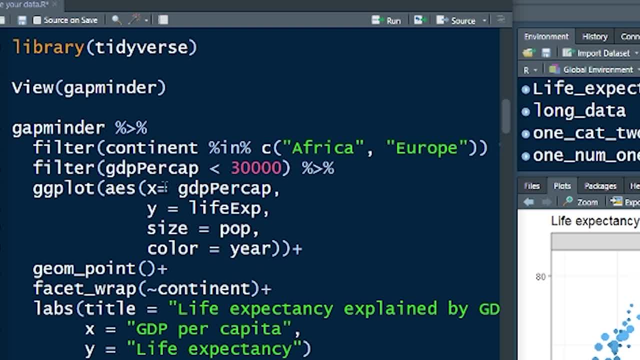 aesthetics and they are now there's. there's four different aesthetics that i'm defining in this particular graphic and we're going to talk about how we deal with the fifth in just a minute. but basically, mapping says for any given variable, for each of the observations in that variable, what. 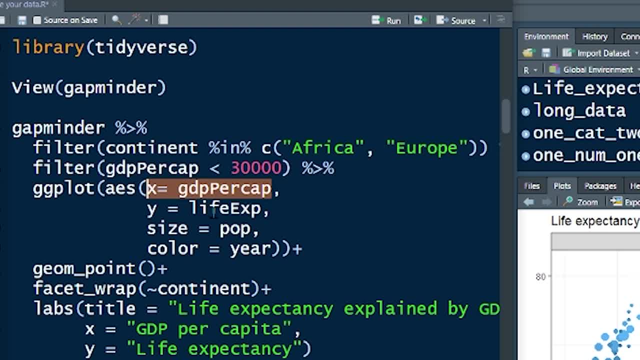 should r do with that observation? what should it connect it with? and we've said, okay, well, the x variable, right. the x-axis, we want that to be mapped out against gdp per capita. the y-axis, we want that to be mapped out against life expectancy. as we plot the different observations, we want the. 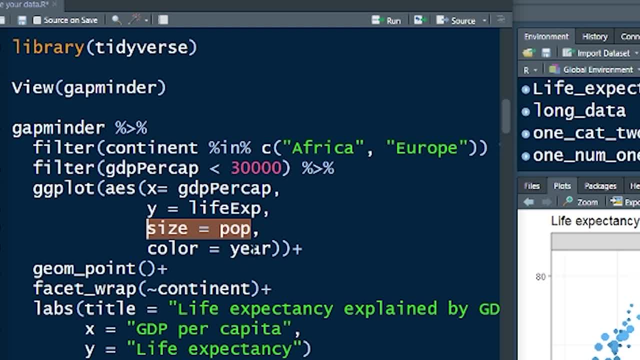 size of that observation to be a function of population size and we want the color to be a function of the year. right, and you can add additional aesthetics in this mapping process. you could. you could say: we want the shape to be a function of something else. you know there's. 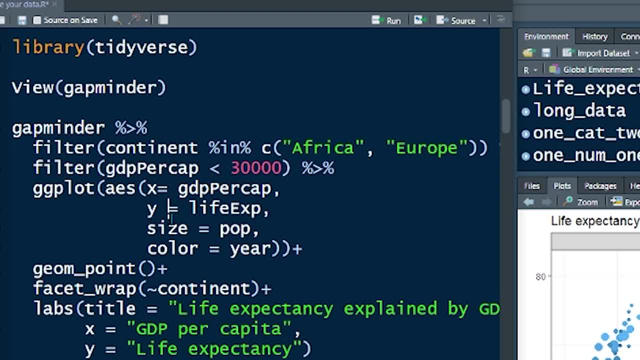 multiple things you can do here. the point is, you want to think about, for each variable that you want to represent on your canvas, what should that variable map out to on that canvas in terms of some sort of aesthetic that you can see, right color, shape, size, uh, you know, there's, there's, there's, lots of things you can do, and so in this case, we've 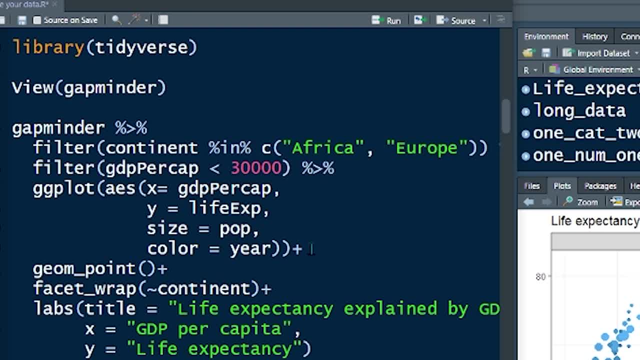 defined those four. these are all numeric variables. right, then we have a little plus that says, okay, we're gonna, we've now, we've defined these things. geom point: this is telling our the next component of our grammar of graphics, which is um the geometry right. and geom point is saying we wanted. 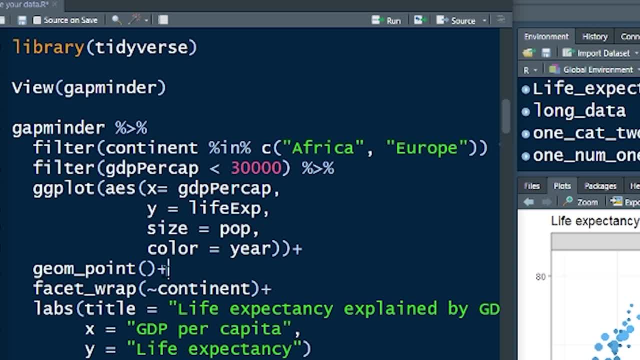 we went r to stick a point or a dot on the canvas for each of the observations. this is where, if this was a history, we could say: we want r to stick a point or a dot on the canvas for each of the observations. this is where, if this was a history, 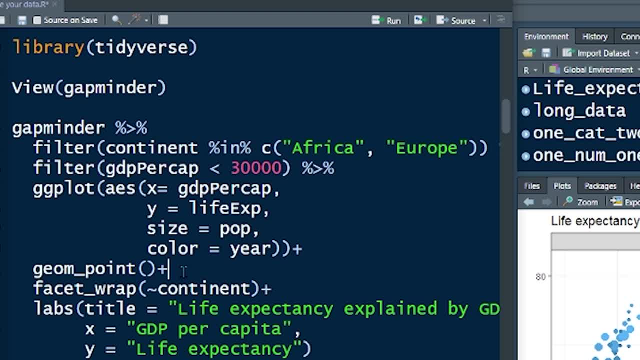 we would. we would tell our: that's a histogram or a bar plot or a density plot or a violin plot, or whatever it is that you want to plot. this is the geometry. this is where you would define that you can add additional information into, into the inside these brackets. right, so that that is uh. 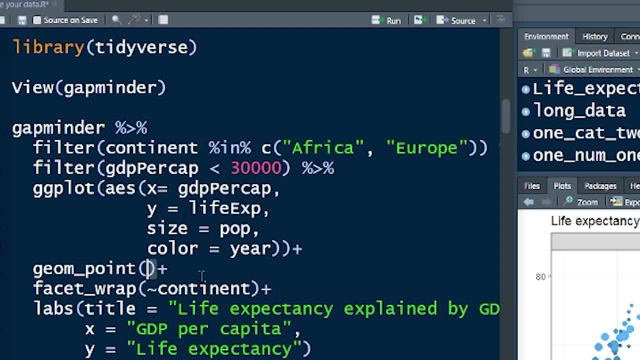 these are the arguments you can put inside there, and sometimes you want to add specific aesthetics into a particular geometry as you layering one layer upon the next, and i'm not going to get into all of that in this video. i have other videos on that that you might want. 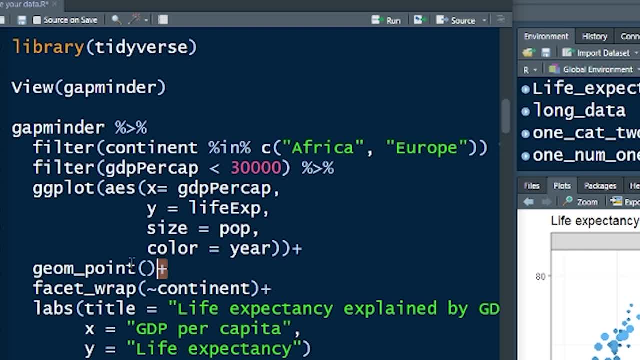 to have a look at. but just to let you know, that's, that's the geometry right there. and then after that we've got an opportunity to do something called a facet wrap, and i've said facet wrap by this little squiggle there is, by continent. so we've said, take all of that data and disaggregate. 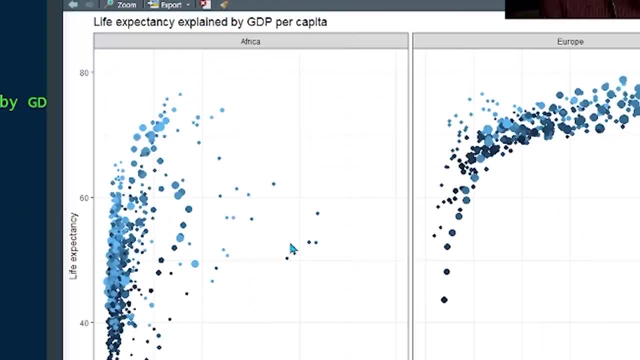 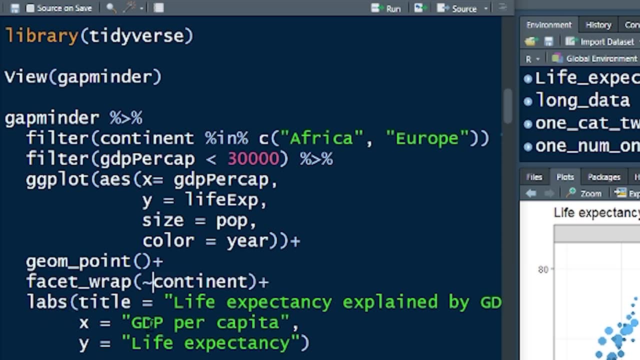 it by continent and it's going to produce this, these two facets over here, uh. and then i've just got labels- labs is for labels- and i've said title, we've given a title. uh, you know, the x-axis give that a label, the y-axis give that label, and we're done right, super duper easy. and if i run that code, 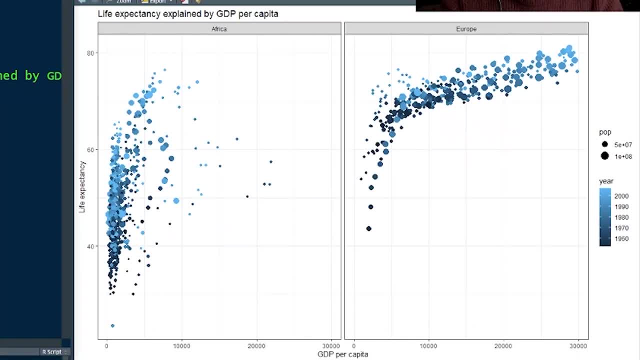 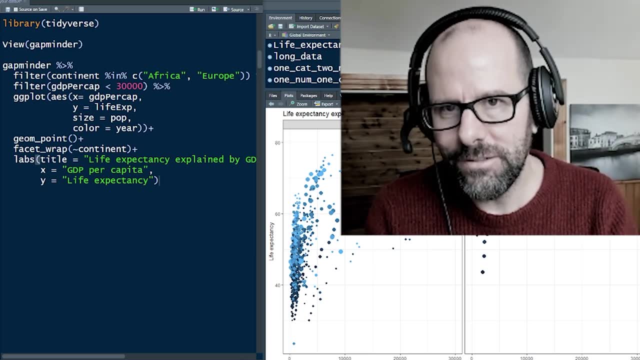 which i've already done. it produces the graphic that's on the screen right now. okay, now, if you want to learn how to create any of these graphics, what you've got to do is practice, right. so download the cheat sheet right click on a link. there should be a link on the screen at the moment. there will. 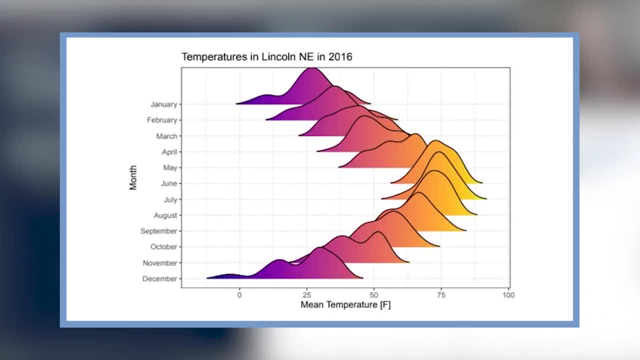 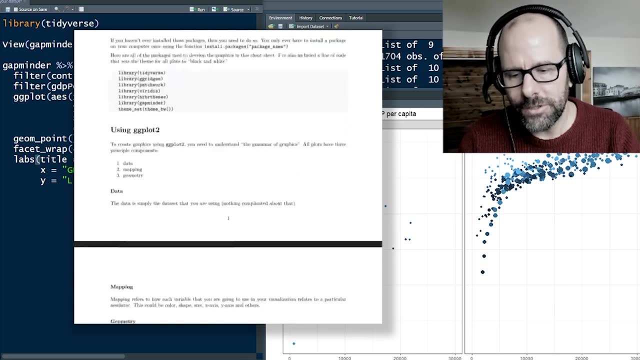 also be a link in the description below. click on the link. download the cheat sheet. go through the code and do it for yourself. replicate that code on your computer. you've got the data. you've got the code. redo these graphics right now. you'll get used to how to do it and you'll be able to apply it then in your own work to your. 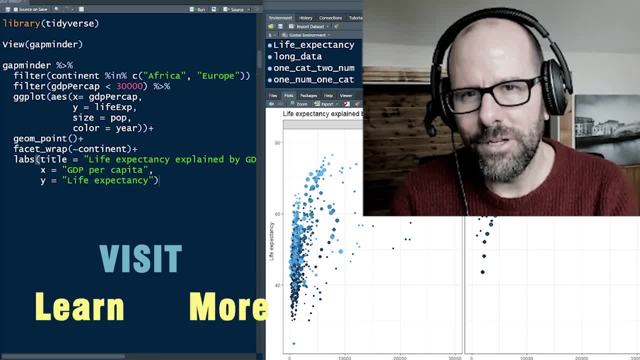 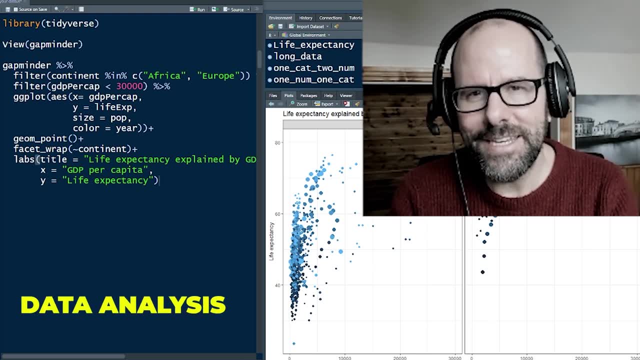 own data. i've got more detailed lessons on how to use ggplot for data visualization at learnmore365.com. now stay and watch the next video on data analysis and if you haven't subscribed, subscribe to this channel. hit the bell notification if you want to get notified of future videos. nice to see. 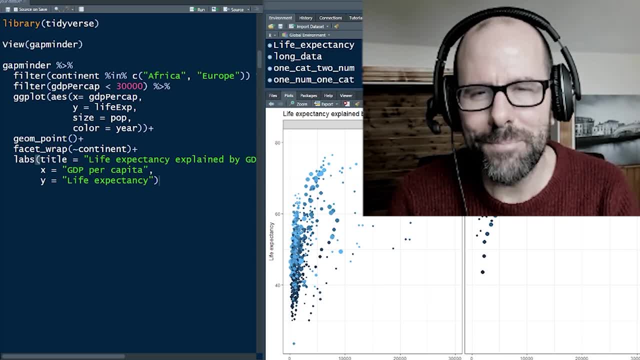 you here, don't ever change, don't do drugs. always your best. see you again soon. take care bye. 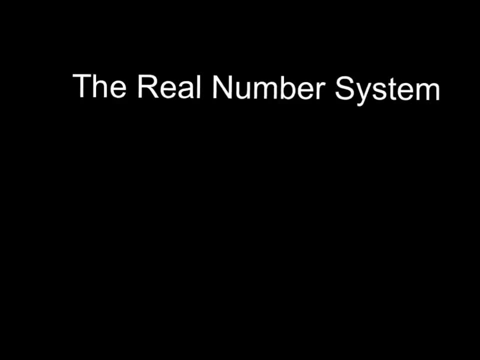 The real number system. In this video you will learn to classify real numbers. Much of this should be a review for you, but we want to make sure that you understand the words to describe different types of real numbers. We will go over real numbers that include rational and irrational numbers, and within the rational numbers we have integers, whole numbers and natural numbers. 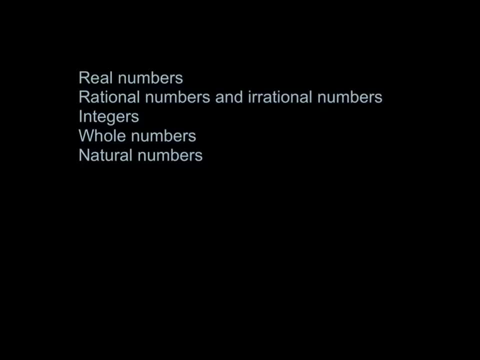 Remember to write the notes down, including the examples, and to make note of any questions you still have. The notes page should be in your notes section And if, at any point, the video is going too quickly, remember that you can pause the video to write down what's on the screen, or you can even replay parts of the video. 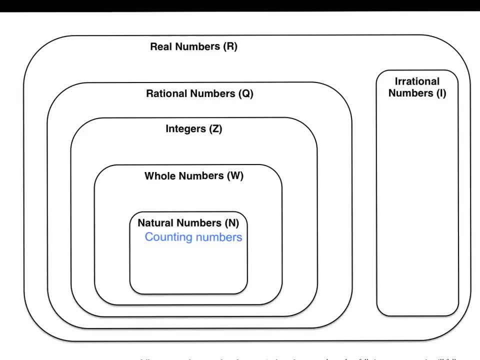 We'll start from the inside out. We'll talk about natural numbers first. Natural numbers are your counting numbers. Those are 1,, 2,, 3,, 4, etc. And that keeps going. Those are the first numbers you learn as a child. 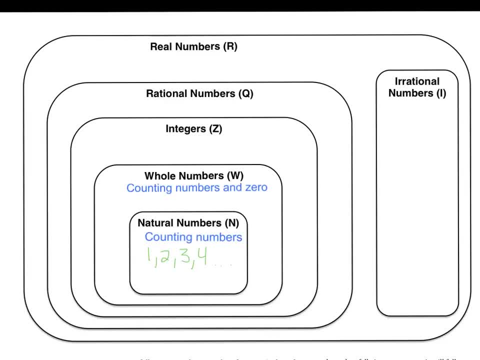 Next we have whole numbers. Whole numbers are all of the counting numbers and zero. So we have 0,, 1,, 2,, 3,, 4, etc. Next we have integers. Integers include counting numbers, their opposites and zero.